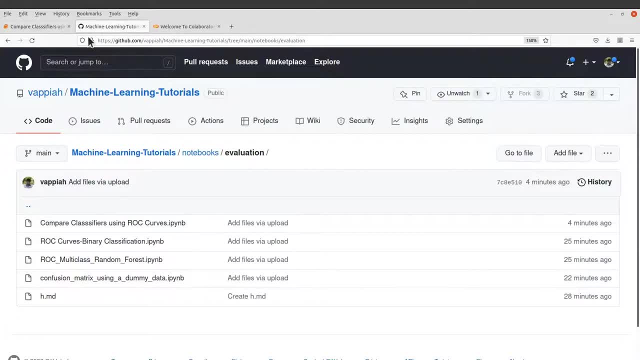 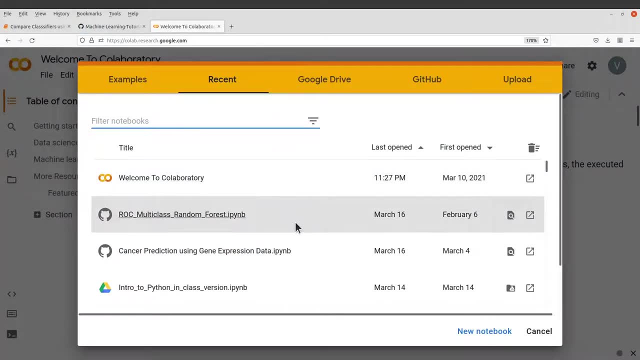 So I have already copied that link, and so what I'll do is to come to Google Colab, which you should also have on your browser login to your Google account. so once you have logged in, you have the Google Collab platform ready for you. so there's a link, and I'll leave this link also in. 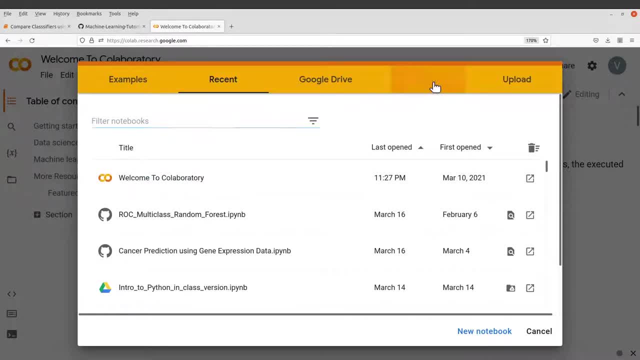 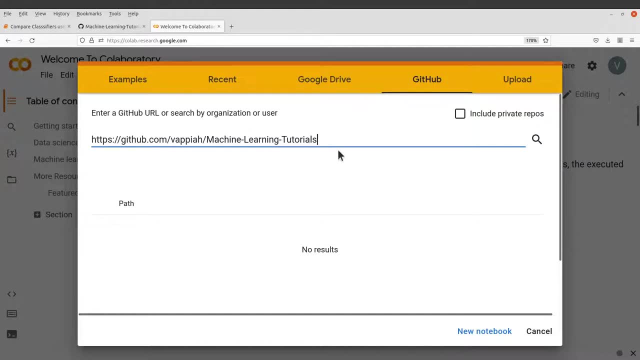 the description box. so here, just go to the github tab and then just paste the link, the github repo link, which is this one here, and then you can search. so once you search, all the notebooks in that repo will be displayed for you. so let's check them out. so let's go scroll down, check notebooks slash- evaluation slash. 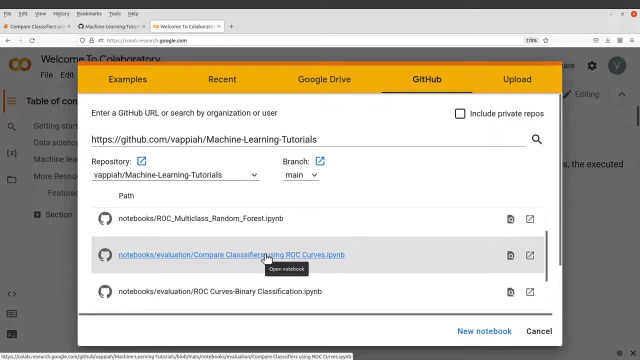 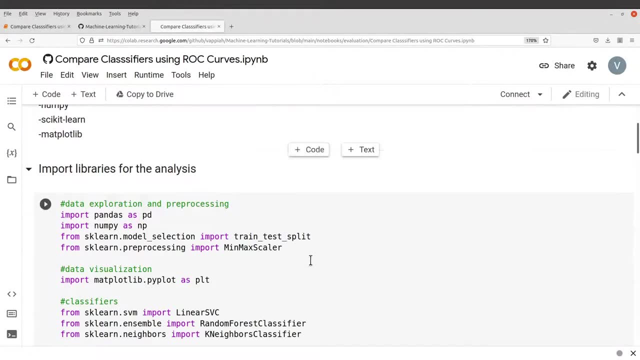 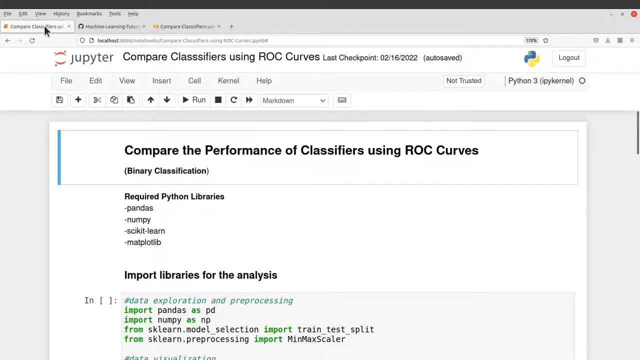 compare classifier. so it should be somewhere here, this one here. so just click it once you see it, and then the notebook will be opened for you here, and so once you are here, you can just run it. I prefer using my Jupyter notebook, so I'll just switch here and then I'll proceed. so we need to first 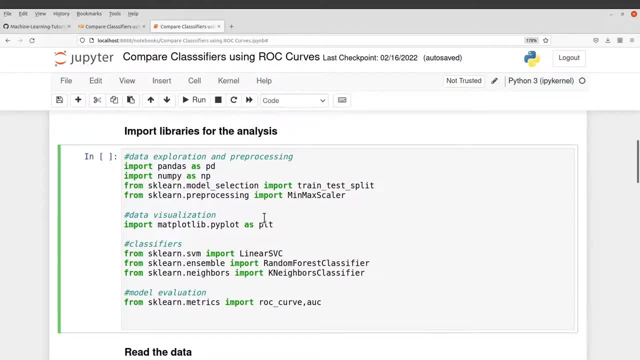 include our computer, and we should be able to set up our computer by opening our libraries, and so let's import them. so we have pandas, numpy. we also have some pre-processing tools, the virtualization library, smartport, lib, and then we have the classifiers and then the evaluation, which is the ROC kernel and AUC. so just 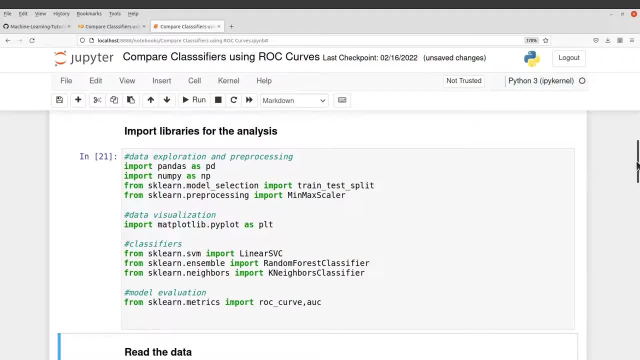 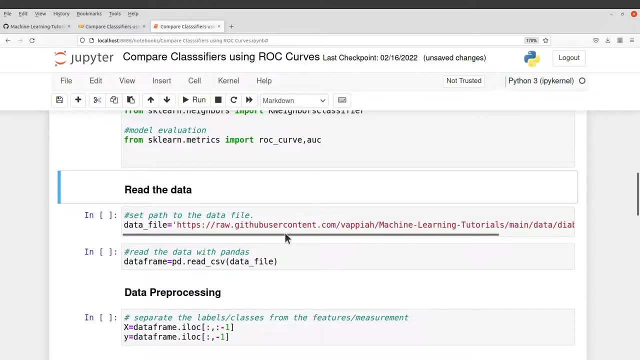 run this cell to get the codes executed. after that, you need to get your data. we need to read the data. I am using the data which is also available on my github page, so the link here is what we need. in case you want the notebook, you can still come to my repo here, the main page, and then just check the data. 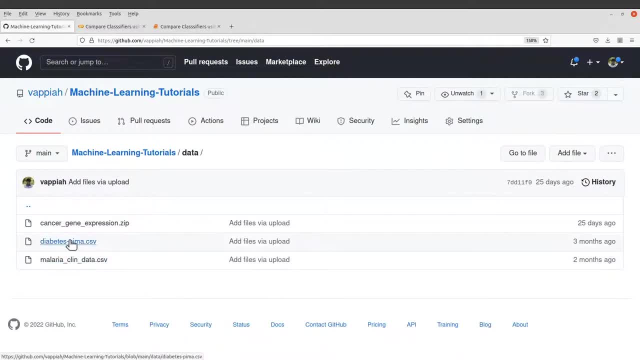 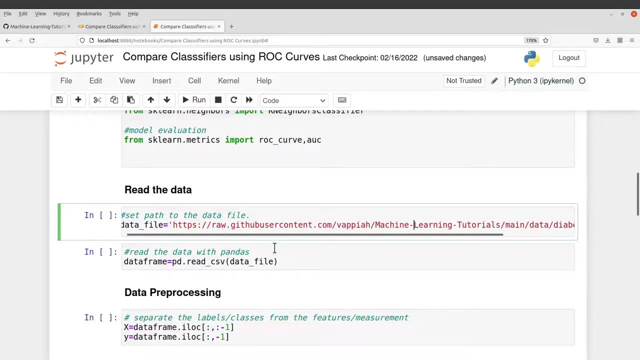 directory. you will see the data there. it is the Pima diabetes data set. it's it's a binary classification problem we are dealing with here. so just take note of that. so just run this cell to get a link and then run this cell again to read the. 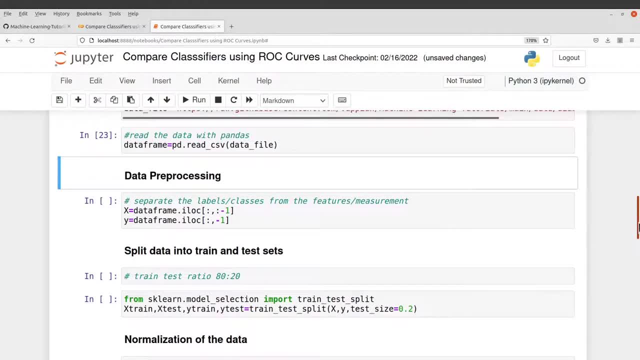 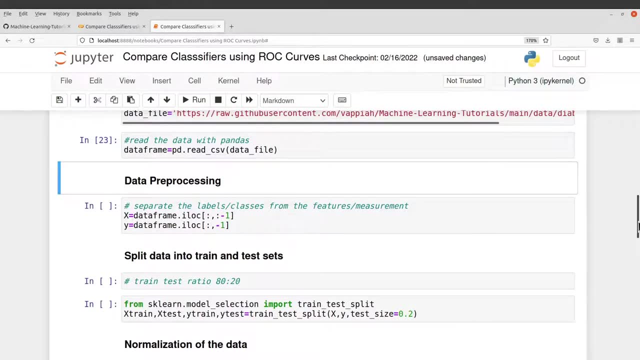 data. so after getting the data, you then proceed with the rest of the activities. with a typical machine learning task, you need to do exploration as well, but in this tutorial our focus is to get the ROC kernel, so I'm going to skip the exploratory parts. so you move straight to the pre-processing. 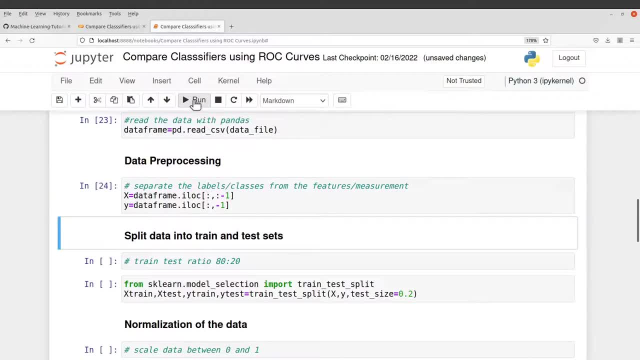 here. so you move straight to the pre-processing here. so you move straight to the pre-processing here to get our data in shape. so this one here, the first cell here, and the pre-processing is to separate the, the values, the variables themselves from the. 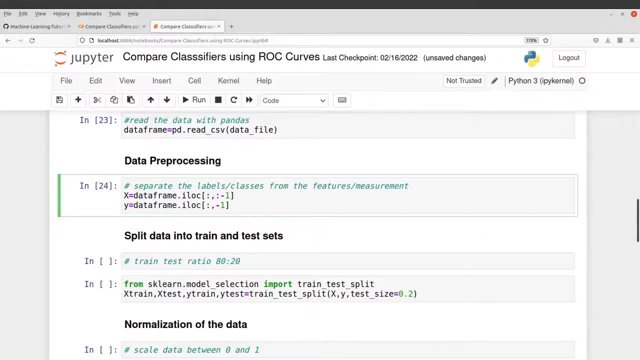 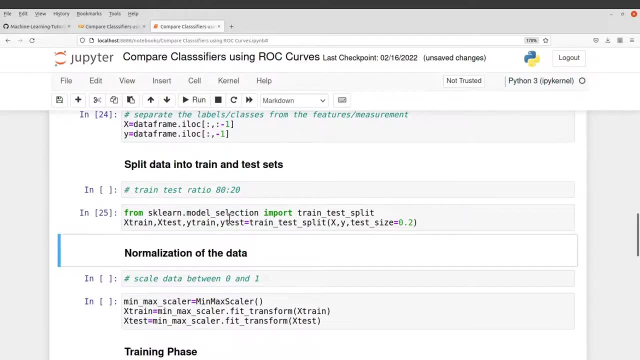 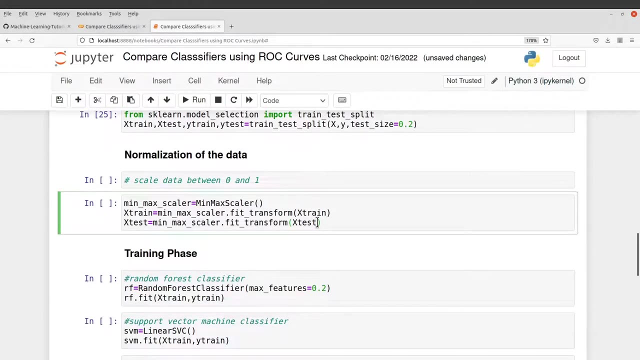 outcome or the class. so that is what this does for you. after that we split the data into training and tested. so we are using 80- 20, so you just split it here, and then we need to normalize the data. so normalization is done so that we can get our values in the same skill if you have values in different skills. 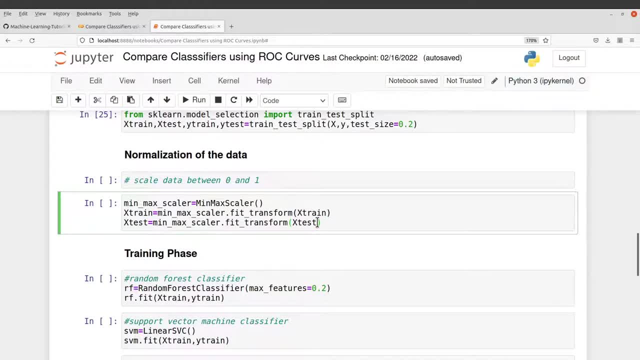 it may affect the models performance. the model may even be biased, so that is why we did it. I'm not the shooter. it can get all of them within the same range. so here the code here will scale the data so that all of them are between zero and. 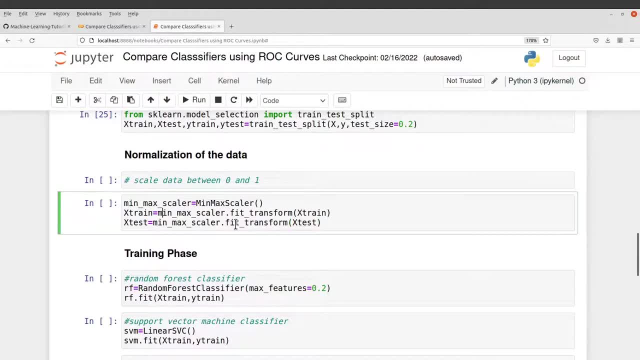 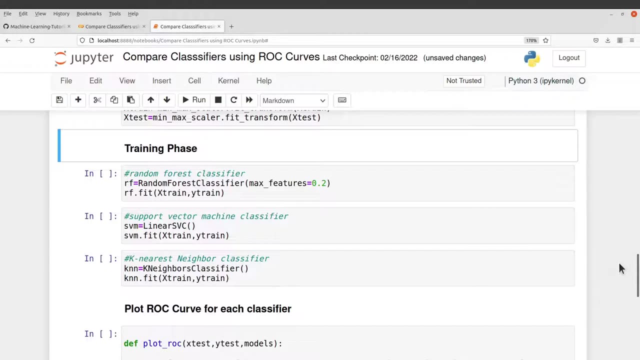 then one. that is what this does for you. if you are interested to go further, you can still do some course, and I'm just very far from here, but I'll skip that for now, so let me run it. it's done. after that, we are going to build the classifiers here, so here we are training them, so we. 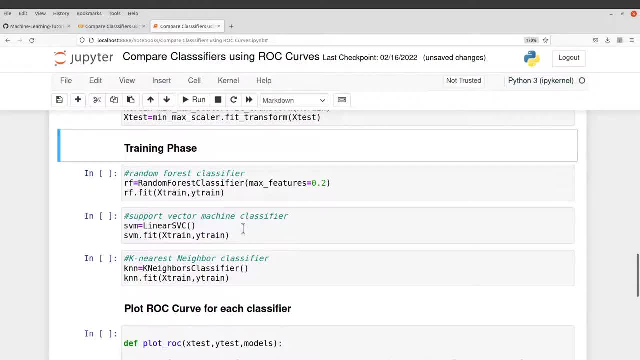 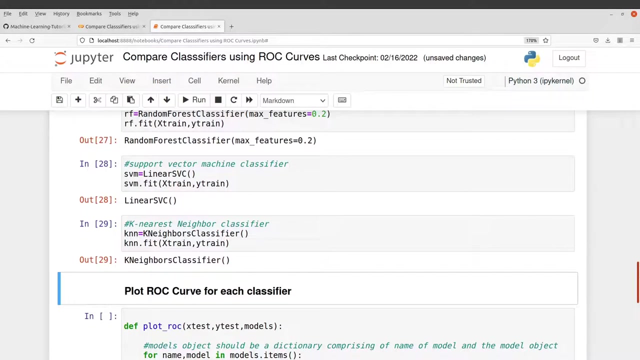 have the three classifier. we have the random forest support vector machine and then k nearest neighbor classifier. so these classifiers are what we are going to use, so let's run each of them here together to get them trained. so I'll run all the three. okay, with IOC curves we need to. 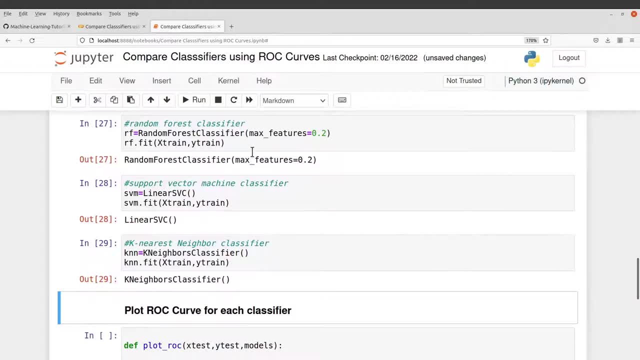 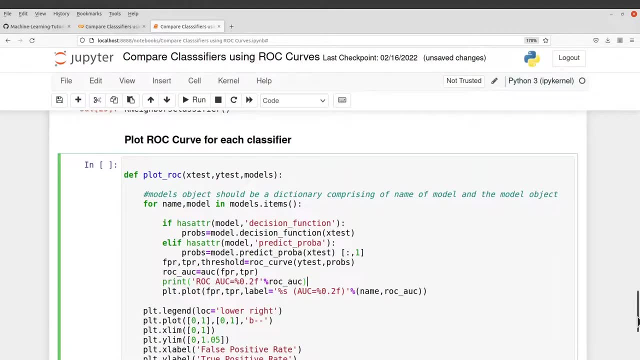 get the probabilities. but because we have three classifiers, I decided to automate the process a bit. so I have created a function here which has everything we need. so the function here: we will get the probabilities and then also generate the IOC curves for us. so let's run this. 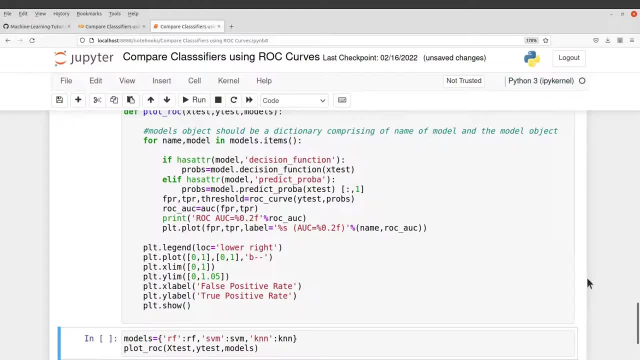 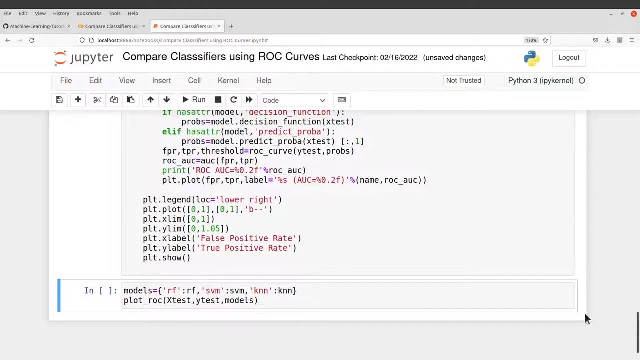 function, so I'll run it and then, because it's a function, we need to call it before it can do the work for us. so that is what this code here would do for us. so this code here has names for each of the models or each of the classifiers, and 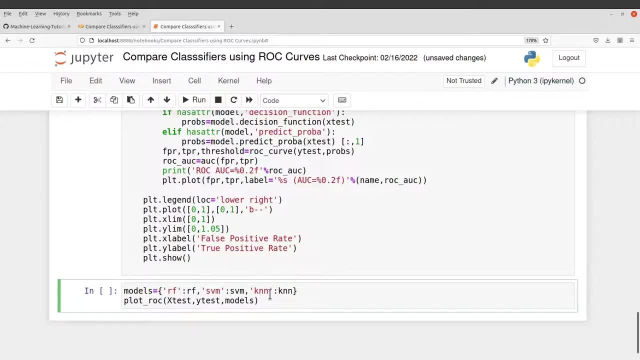 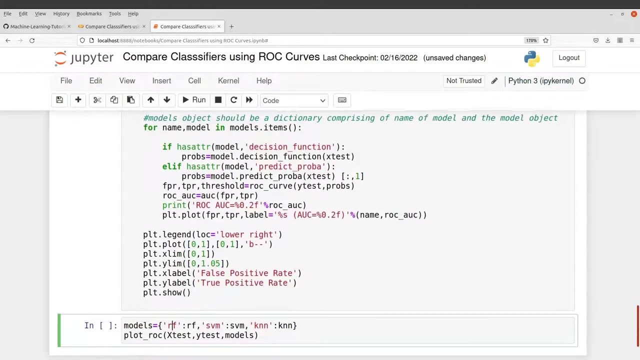 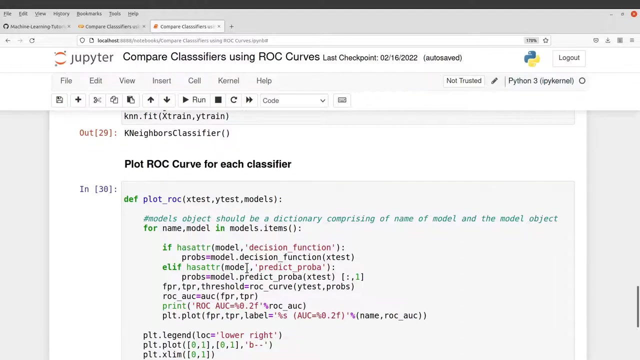 then it calls the function and also specify the models themselves for us, I mean the model objects. so that is what we have here and so, yeah, the dictionary here is applied. and so what happens is that the function here will take the dictionary and then will iterate over the values in the 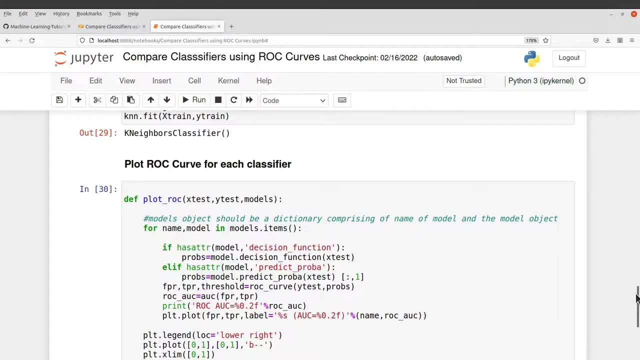 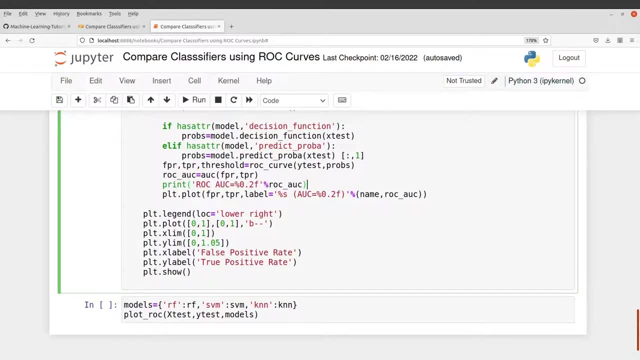 dictionary and then use that to process and then get the IOC curves for us. so everything here is a bit automated for you. so just so that beginners like you can also quickly get your hands dirty with data science and then model evaluation. so that is why I've made it this simple. 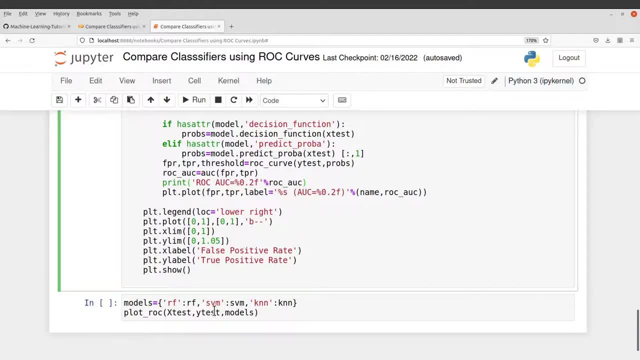 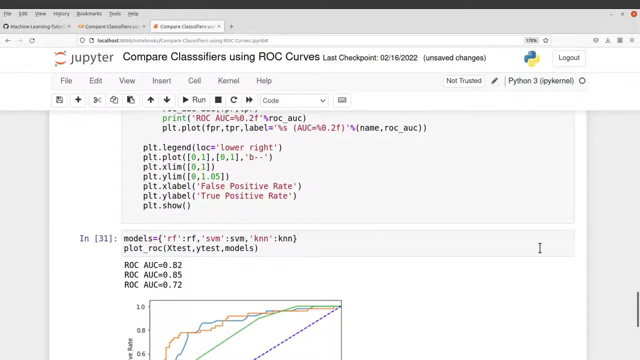 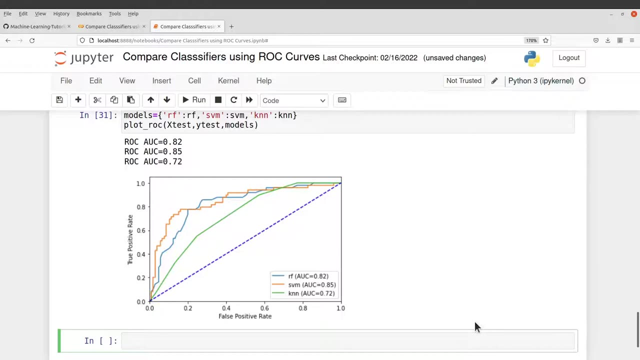 so let's run this code to get the IOC curves. let's check it here. okay, perfect, so the IOC curves have been generated on the same figure for us, so now it becomes easy to compare. so we have different color codes for each of the classifiers. so we have 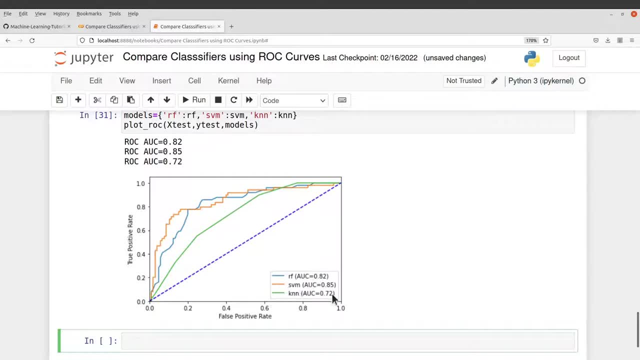 Rf, which is random for us, SVM, and then KNN, and so here are their IOC values here. so you can see from here that SPM has the highest IOC score or AUC value. so this means that in terms of the performance, if you are using 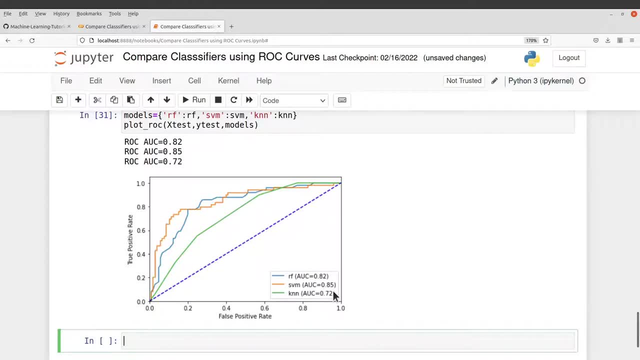 the AOC values to evaluate and see if a model is good or bad. SVM is the best performing model here. that is why it has 0.85SVM, is followed by RF, which is random forest, which is 0.82, and you also have KNM, which has 0.72. so 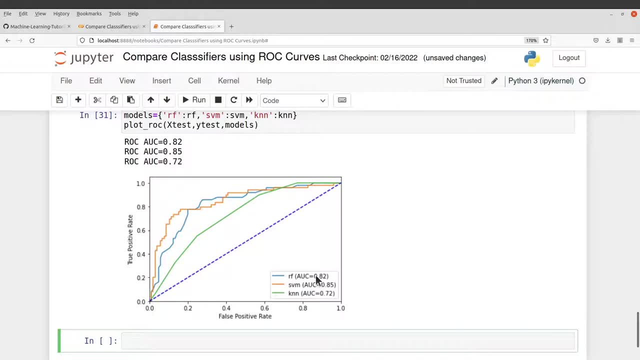 among these three the best is SVM, and then it's followed by RF and then the least performing model is the KNM. if you don't have the values here, you can still use some properties here to also understand and get the performance of the models. so for the IRC curves you can use the steepness.